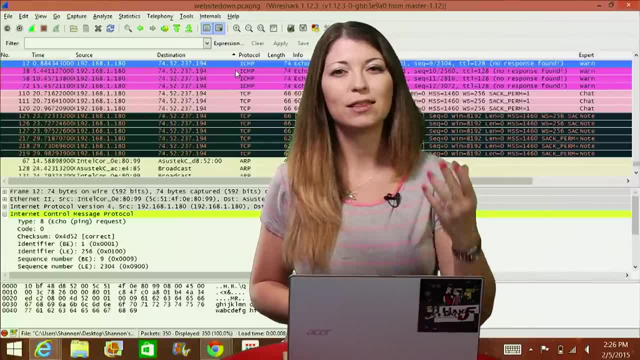 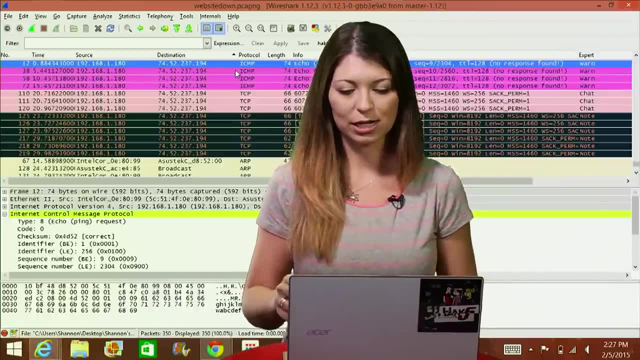 very obvious to tell. Once we get those four requests we can then try searching for it in the browser. If I do that, I get a bunch of synchronized packets but no answers to these. You'll notice up here I also have all these TCP protocol packets. Now those 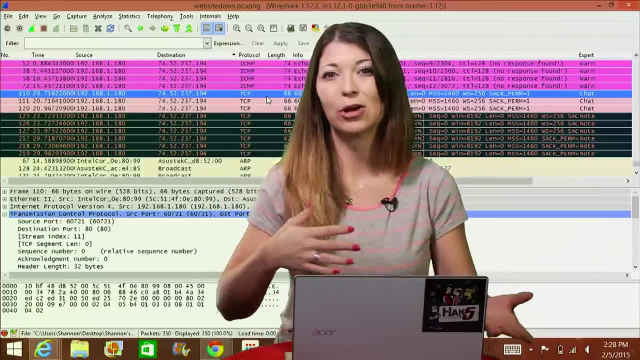 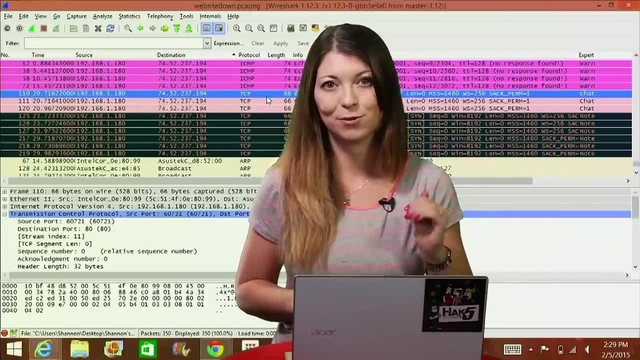 happen whenever you search for it in the browser and you end up getting that error code. I would get a bunch of synchronized packets but no answers. So it keeps on trying to retransmit up to three different times. Now you see a whole bunch of transmits down here as well. 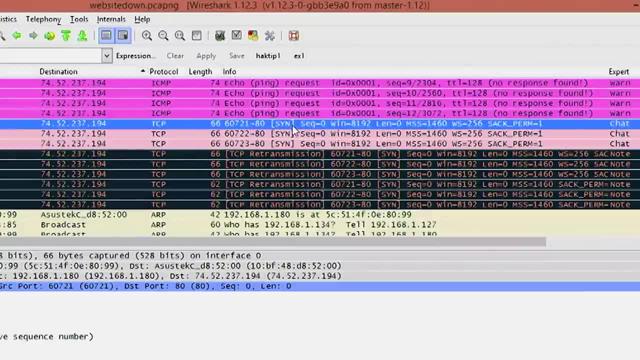 So we have the TCP protocol packet- port 80, synchronized, But when it can't synchronize, it tries this TCP retransmission, And this is the same thing. So I have the TCP protocol packet- port 80, synchronized, but when it can't synchronize, it tries this TCP retransmission, And this is the same thing. 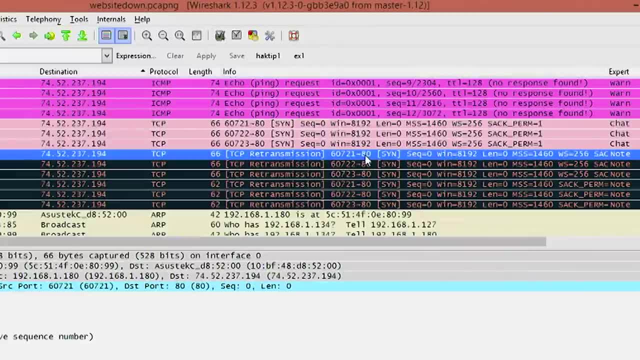 that I have the TCP protocol packet- port 80, synchronized. But when it can't synchronize, This is also TCP protocol and it tries the same exact thing. You'll notice that these two- I believe it's these two- match up with this one and then 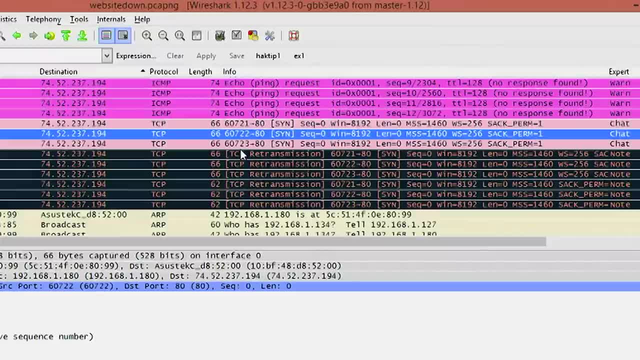 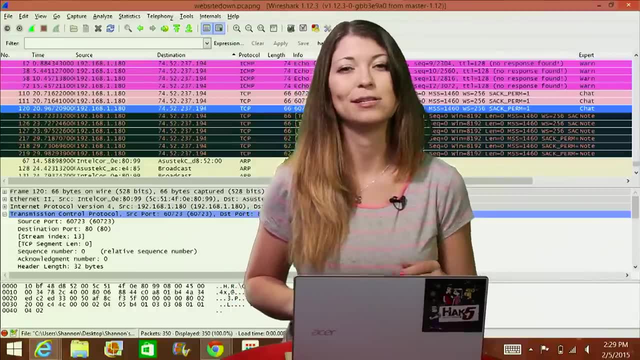 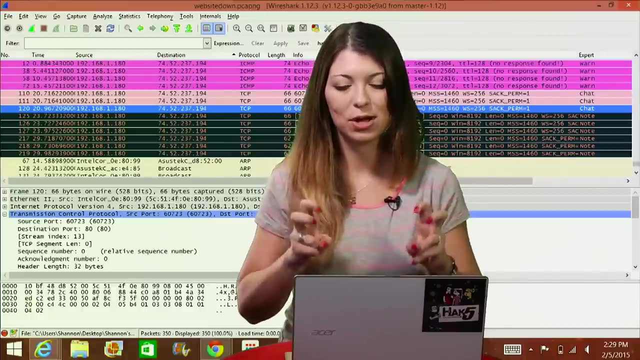 below that we have a second one that matches up with the second two TCP retransmissions. The third one matches up with these because it's going to try three times and after that it's going to basically come out with an error. If you take a closer look at the info dialog, the ping requests all say no response found. 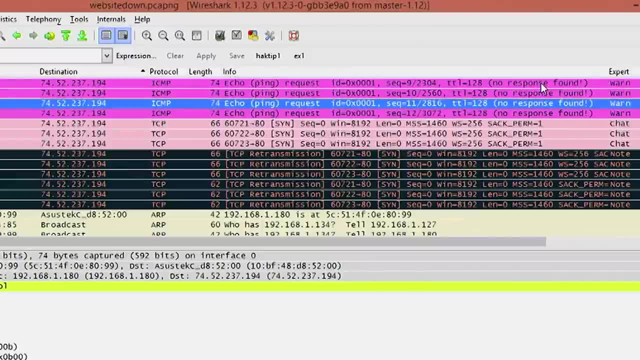 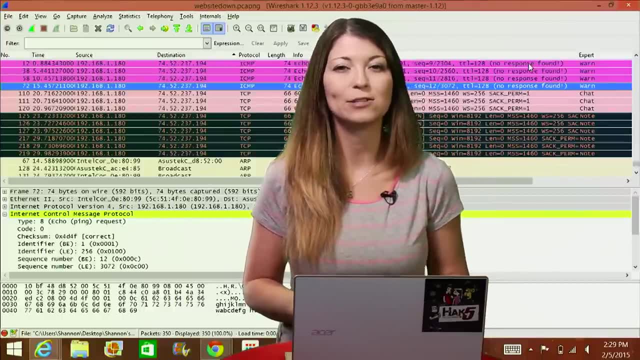 That's kind of interesting. if we look all the way up here, all four of them say no response. found Very, very easy way to tell if there's an error going on while you're trying to visit a website While the TCP packets just say retransmission. 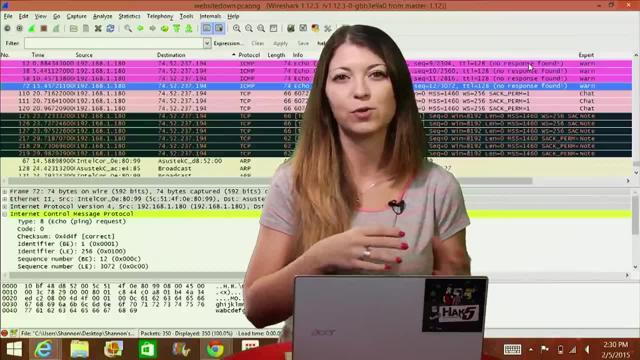 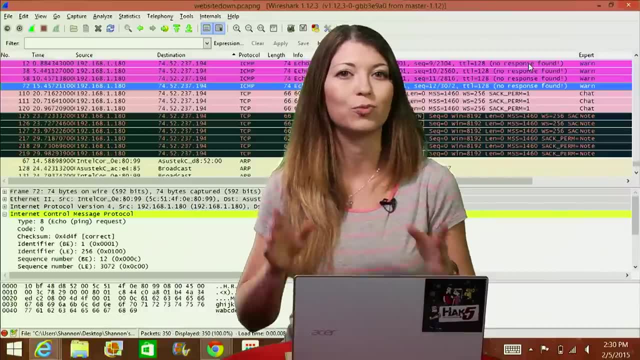 If we look at other packets in this capture for other sites within my network, we can prove that the problem only occurs when trying to visit this one site, not the entire network. We know that it's an issue with this website, not everything else. 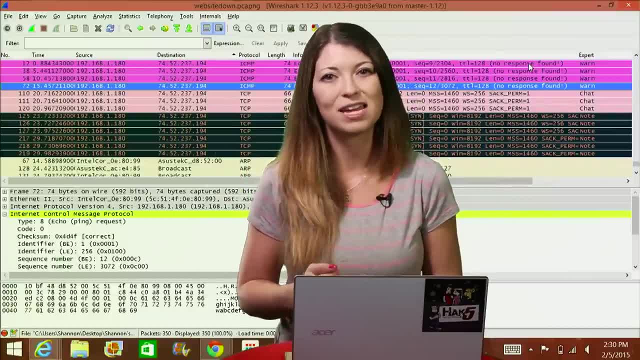 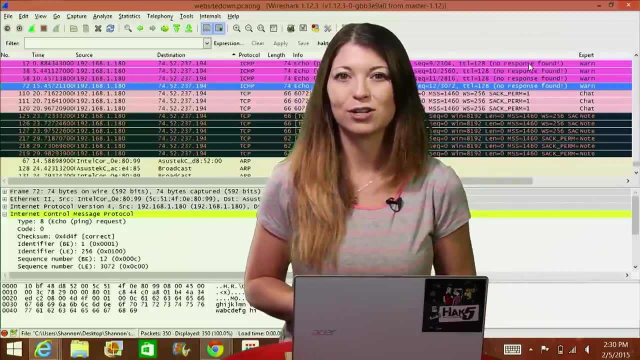 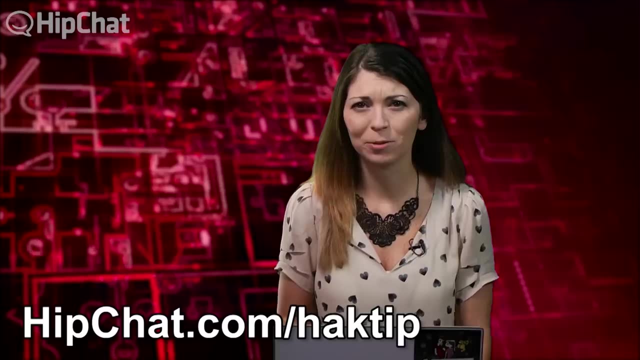 After the break I'll detail a few other problems that you might face If you're dealing with issues trying to reconnect to the internets and whatnot, and what to look for in Wireshark. How is your team communicating? Are they using a variety of email, IM, texting, cloud storage and document sharing apps? 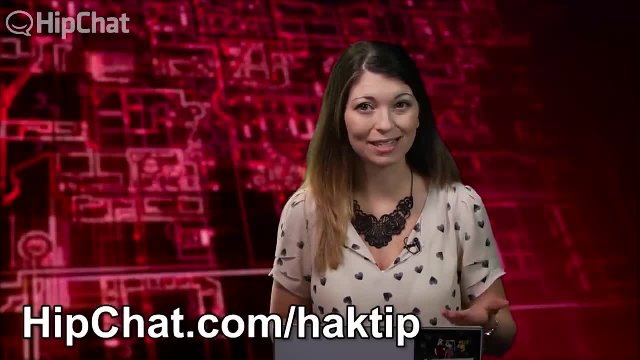 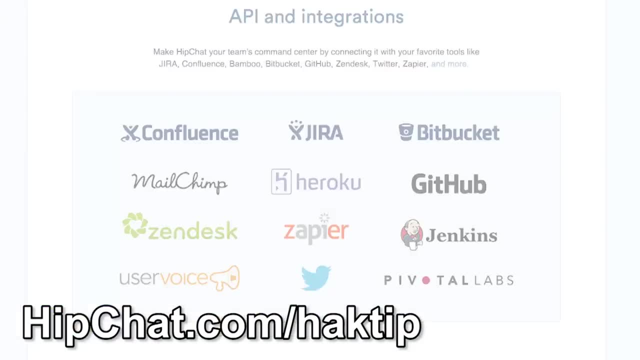 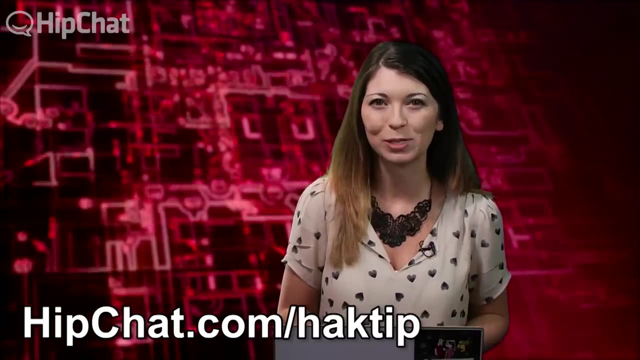 HipChat puts everything in one place and is designed specifically for businesses. This solution called HipChat is IM, video chat, document sharing, screen sharing system, updates, code sharing, integrated into one simple platform. Email is too slow, Meetings get sidetracked and regular IMs just don't work well for groups. 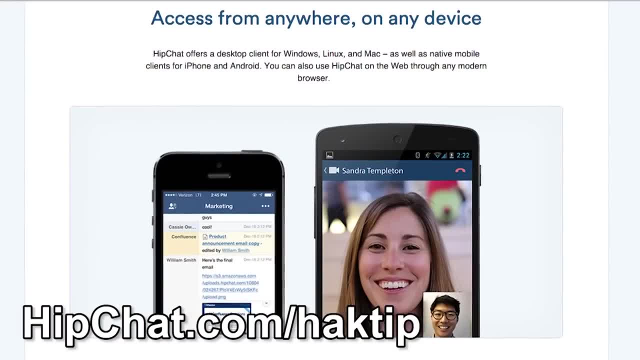 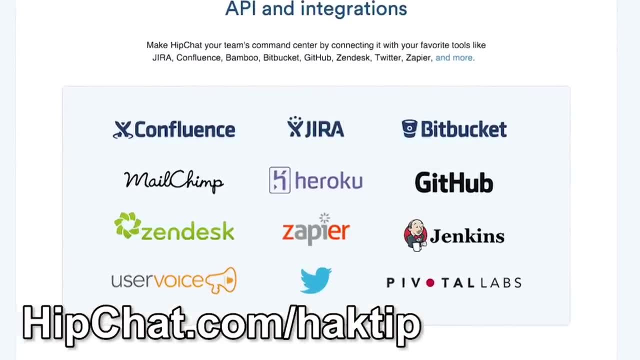 HipChat keeps your team in sync and it works on any device, no matter where you are. And the best part, HipChat is integrated with the top developer tools like GitHub, which is my favorite, Jira, Zendesk and more. 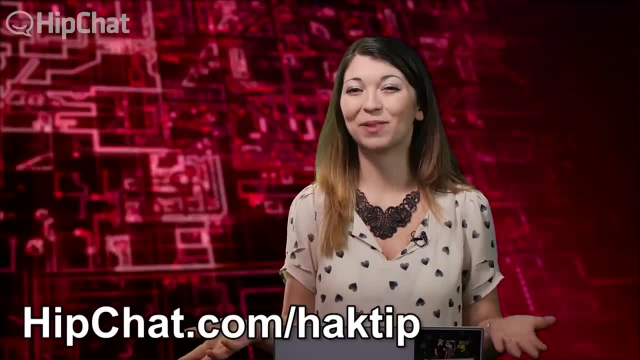 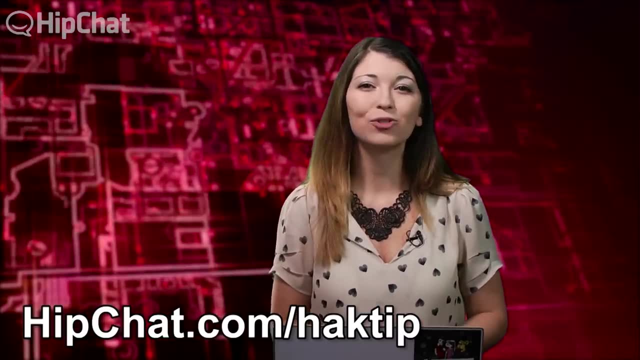 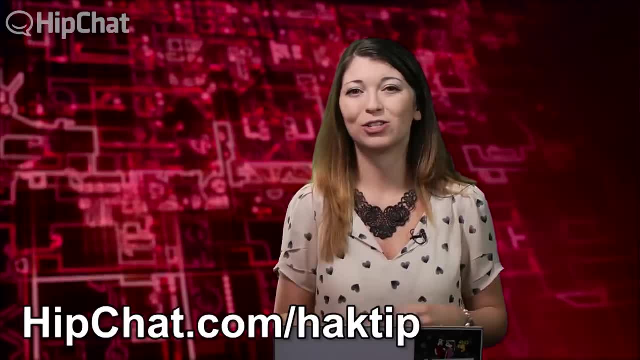 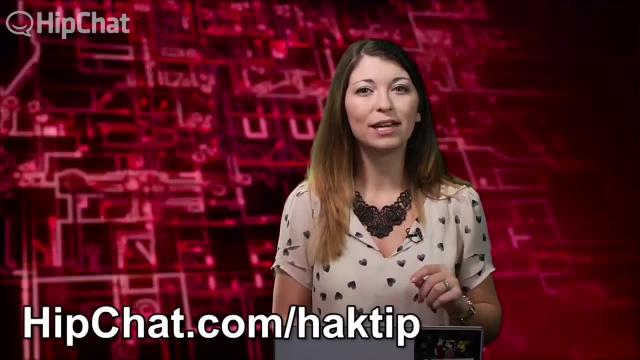 I'm also sending Darren little code snippets for my stuff on Hack5.. All that Arduino code is super simple to send my GitHub account. There is also a freemium version which you can use for free forever, but for the next 30 days you'll get the full version of HipChat for free, which includes the bonus features. 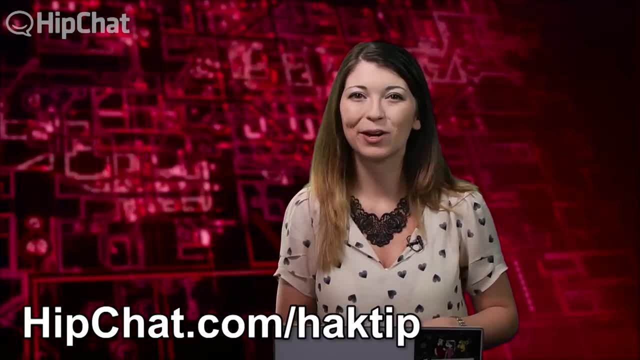 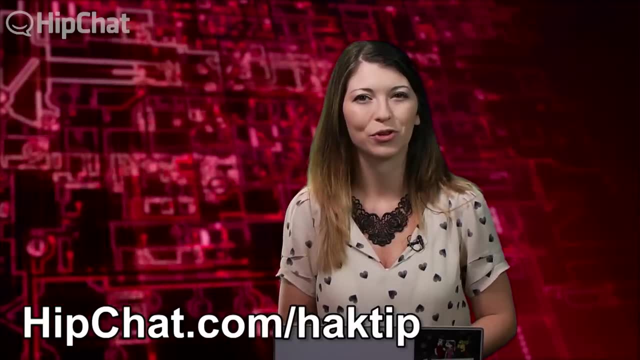 of video and screen sharing. You can try HipChat for free, no credit card required. Visit hipchatcom. slash hacktip. sign up. click on start chatting, then invite a few team members and try it for free for 30 days. 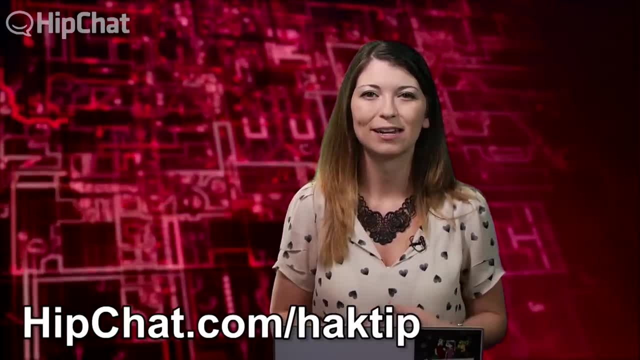 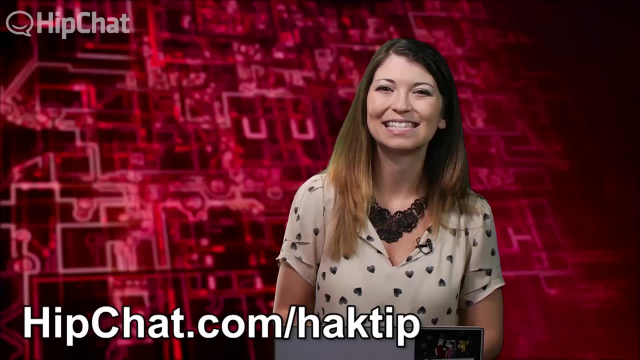 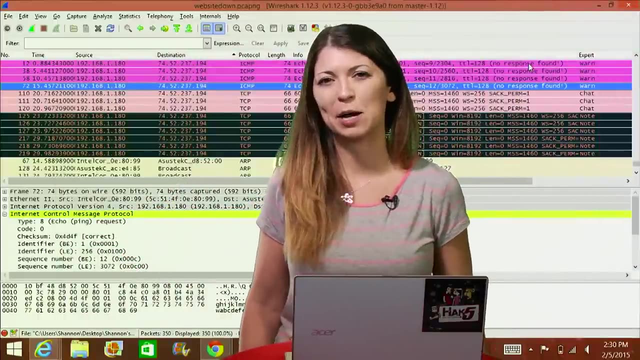 Remember that's hipchatcom slash hacktip And for the first 100 signups, HipChat is going to extend their 30-day free trial offer to 90 days. HipChat, your team, your project in sync instantly. We are back with more disconnection, failures and sad times in Wireshark. 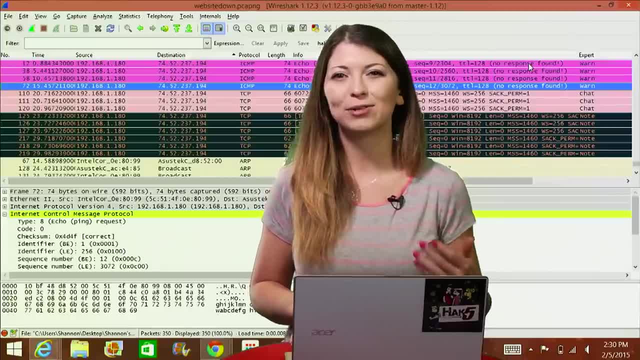 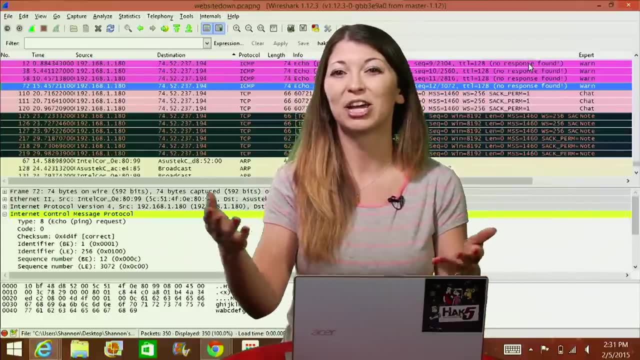 Okay, they're not too sad if you can solve the problem. Now we know how to see if a site is down in Wireshark, but what else can we figure out? Because there's a lot that we can probably figure out. I've run into a problem where I couldn't access the internet, but all of my coworkers 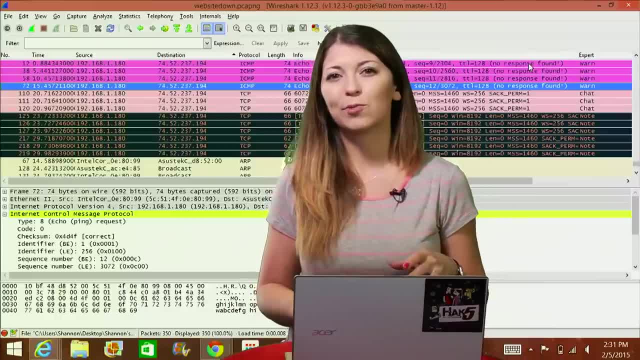 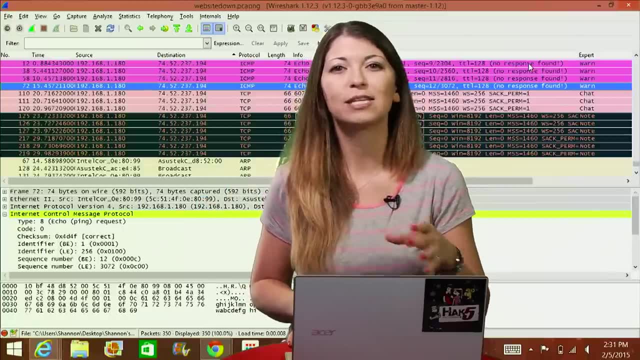 could, for example. This is a great one. So we used a single router and the IP addresses all came from DHCP. This actually happened at the Hack5 warehouse. Now, by using Wireshark, I was able to determine that the problem was with DNS. 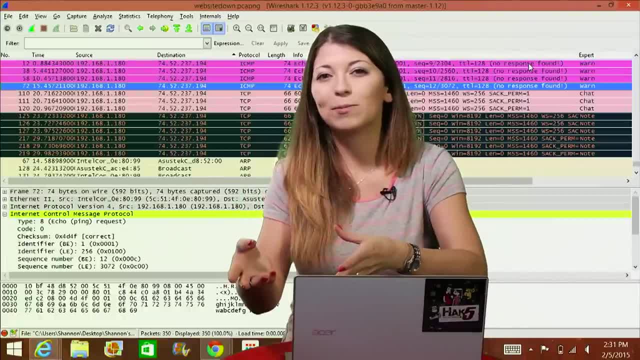 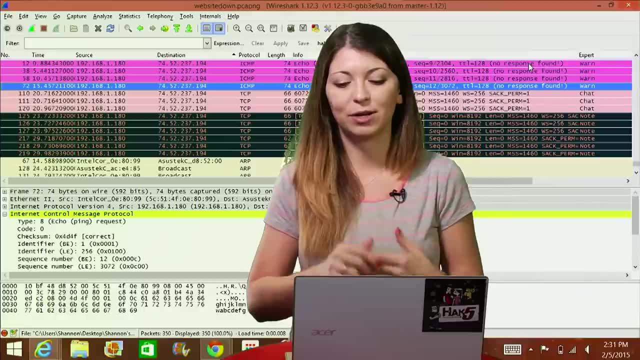 I was able to reach my router and my computer had no problem connecting to it, but couldn't figure out the DNS request. Everyone else could log onto the internet, so I knew it must have been a problem with my computer itself. We were able to find the problem was because I had to manually set my default IP address. 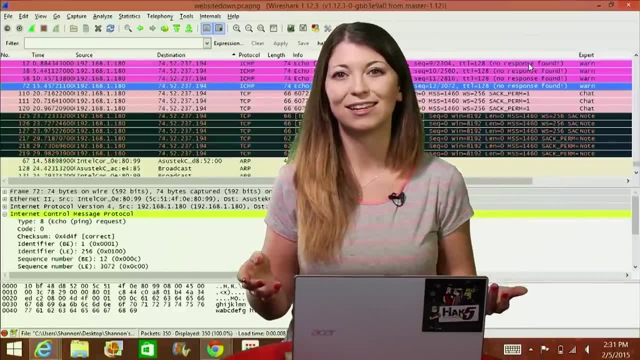 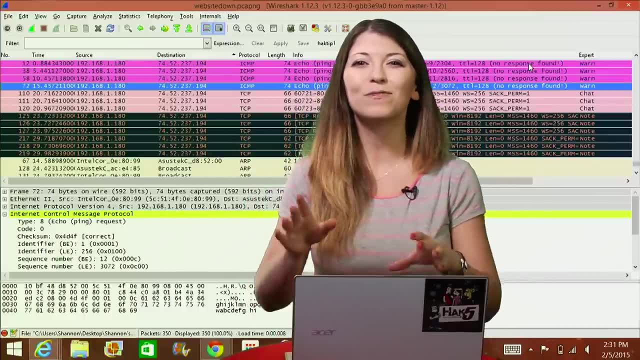 to a default gateway address instead of letting it be DHCP assigned. So I switched it back and then, ta-da, it worked and I could totally hit Google and get on my Facebook. Now what if you can access the net but you keep getting a can't display webpage? 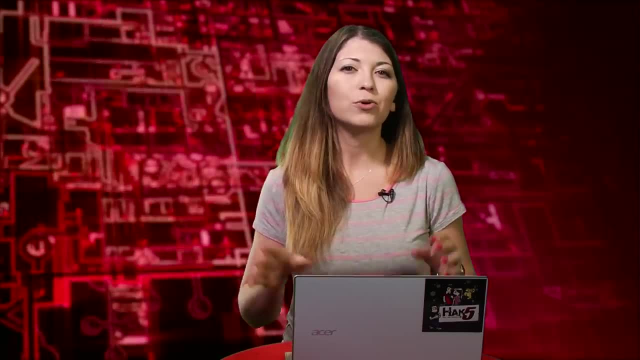 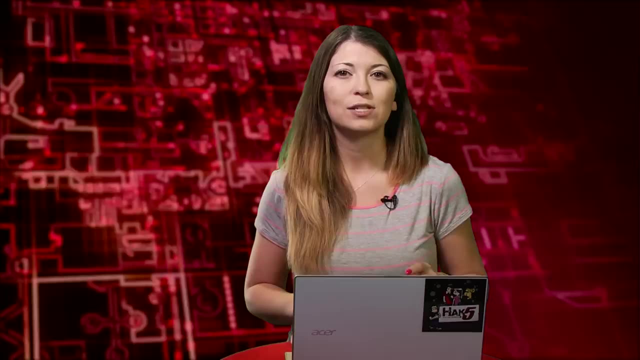 We hate those errors that shows up on your browser. If you are in a really small network, such as here in the Hack warehouse or wherever you might be, and you pull up Wireshark, this would show you sending the site a TCP packet. 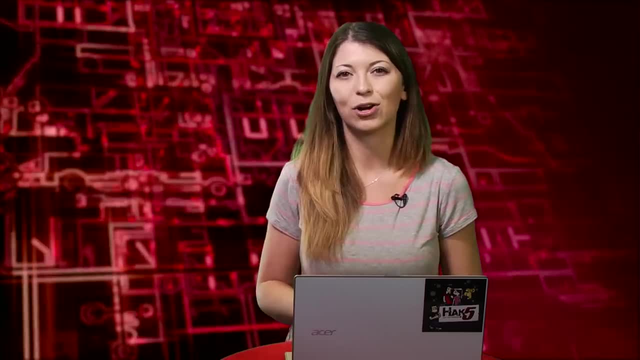 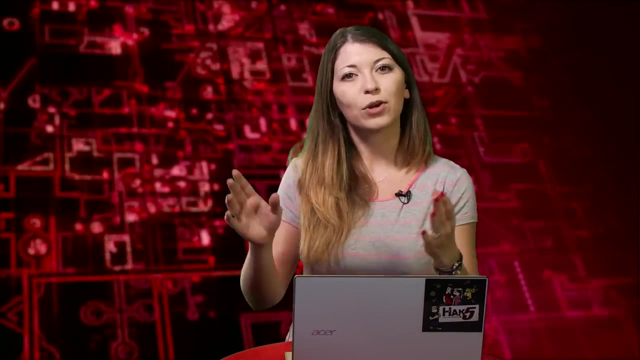 but you would end up getting an RST error or reset packet error back to you. That packet terminates the communication and after a few seconds the browser gives you an error If you are able to send a TCP packet through your router to the net, but you have trouble. 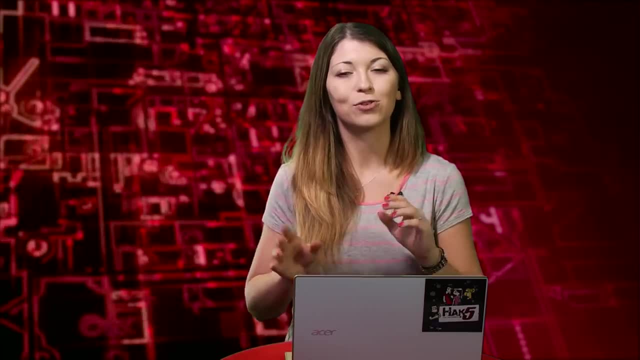 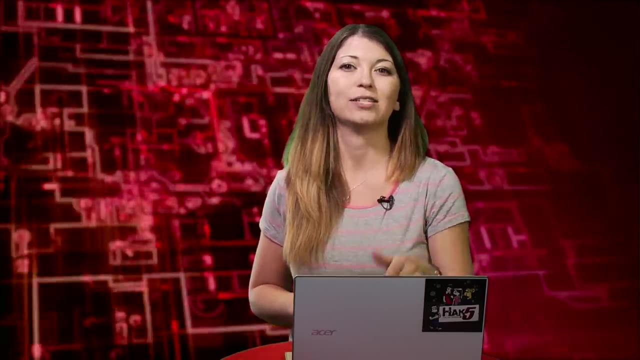 sending a DNS query. it could be because the host file for your device already has the DNS mapped to that IP, or because it's mapped in the DNS cache. So what you would do at this point is check your computer's host file for the easiest. 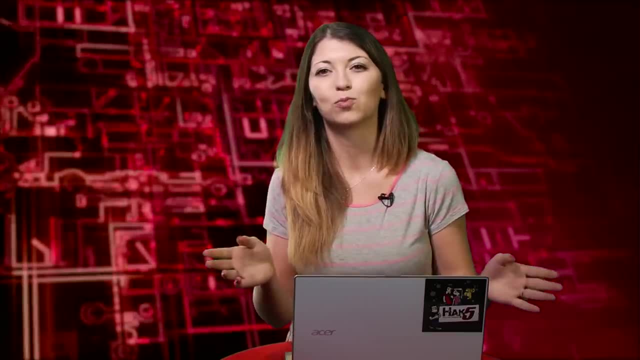 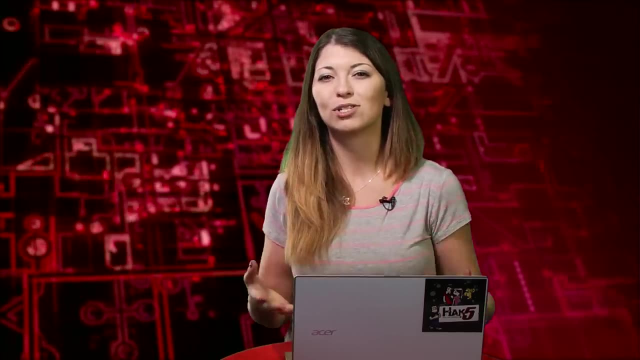 solution Which would, Which would be the easiest solution, and then just remove the DNS mapping if it ends up being there and it's incorrect. By checking Wireshark for these kind of issues and understanding the packets, you can then fix all sorts of problems faster for your network and for your coworkers, or for even. 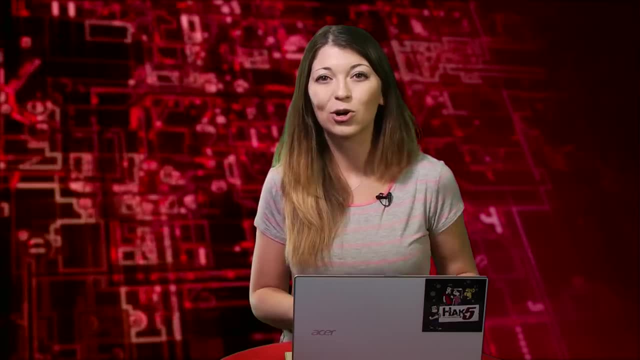 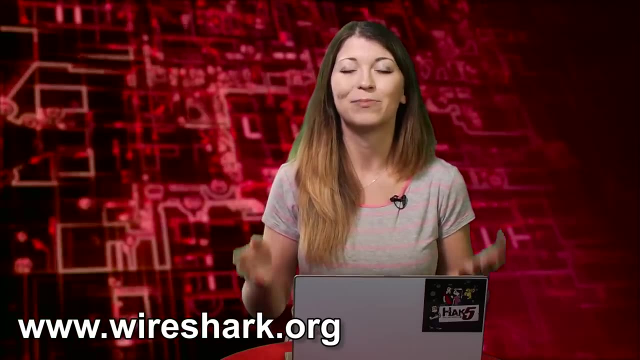 just your friends and family. There are a ton of other problems that can occur when trying to establish a connection to the outside world, so read up on some of the examples online and on the Wireshark website, because there's tons of them. They're really, really good examples. 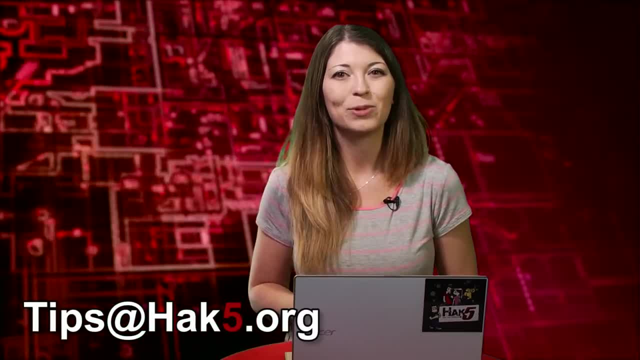 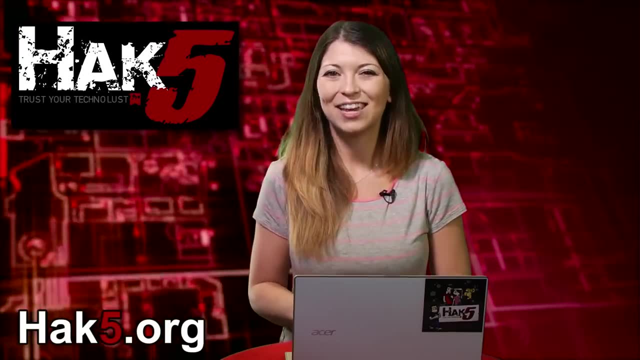 Of course, let me know what you think as well. You can send a comment below, or you can email us tips at hack5.org. and be sure to check out our sister show Hack 5, for more great stuff, just like this. 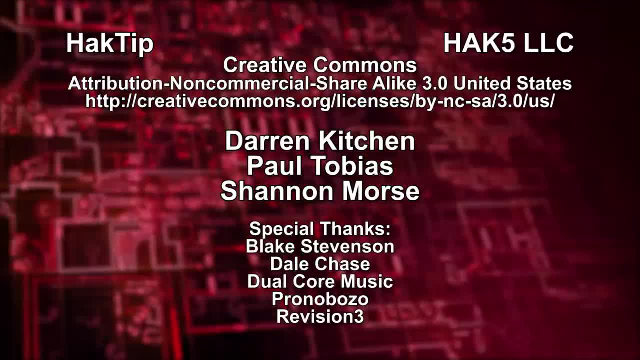 I'll be there reminding you to trust your technolust. Woo, one takes nubs.